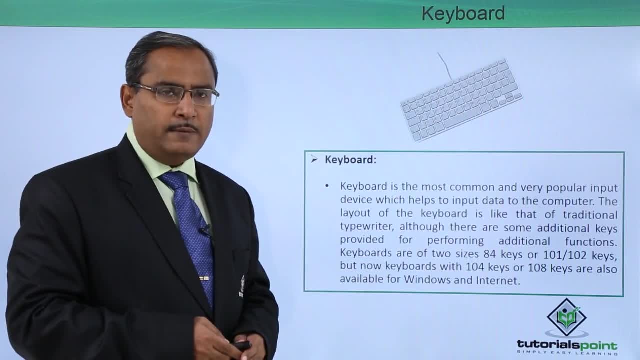 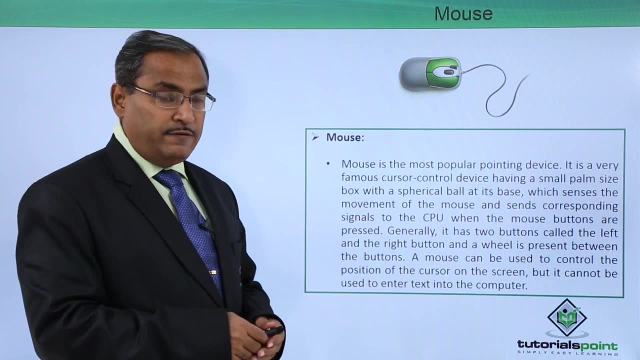 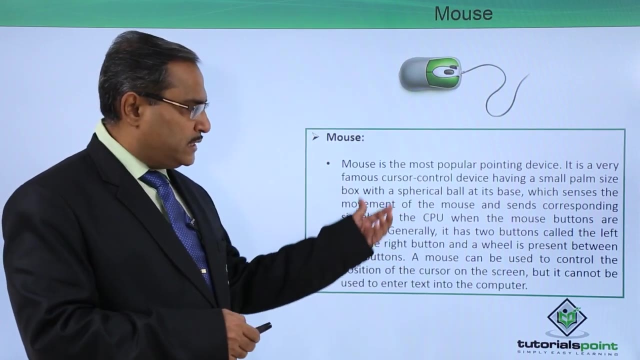 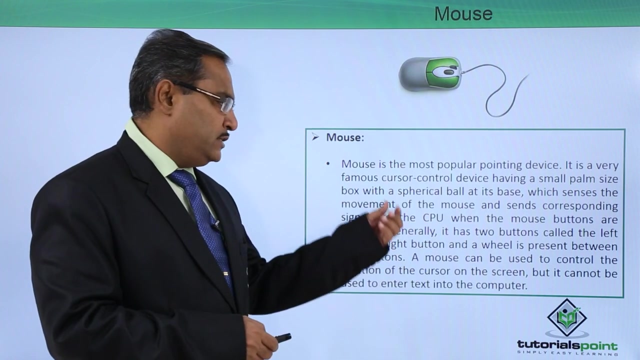 keys for the control of the multimedia base files. Now we are going to discuss mouse. So mouse is the most popular pointing device and it is a very famous cursor control device having a small pump size box with a spherical ball at its base which senses the movement of the mouse and sense corresponding signal to 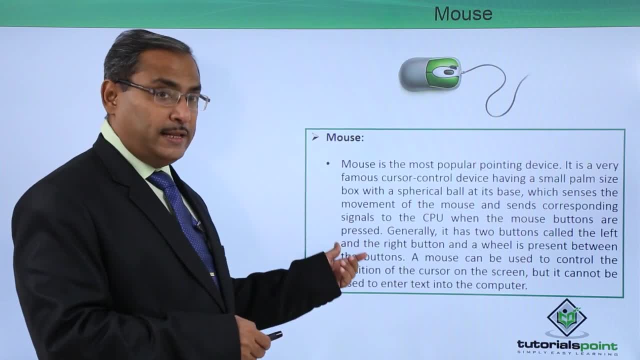 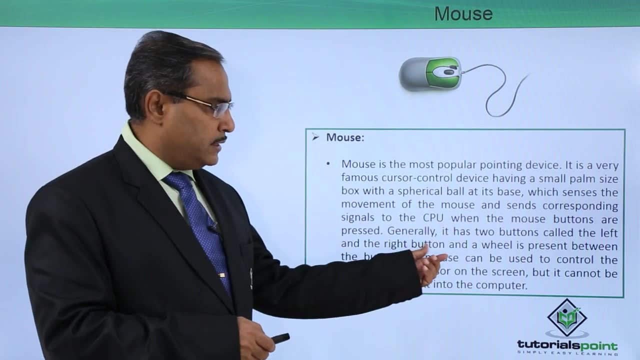 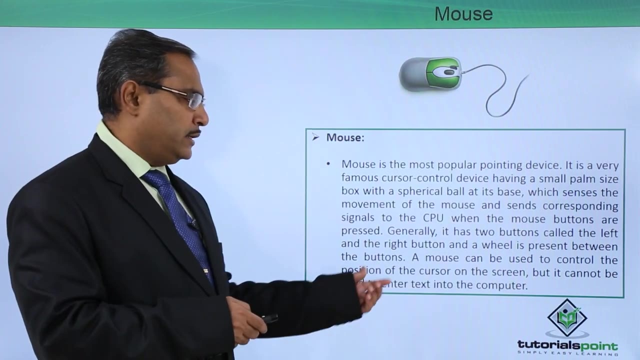 the CPU when the mouse buttons are pressed. So generally it has got two mouse buttons, So one is a left button and the other one is known as a right button and that is a wheel which is present in between these two buttons. A mouse can be used to control the position of the cursor on the screen, but it cannot. 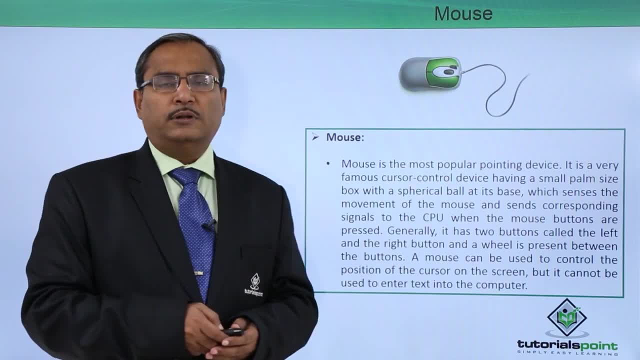 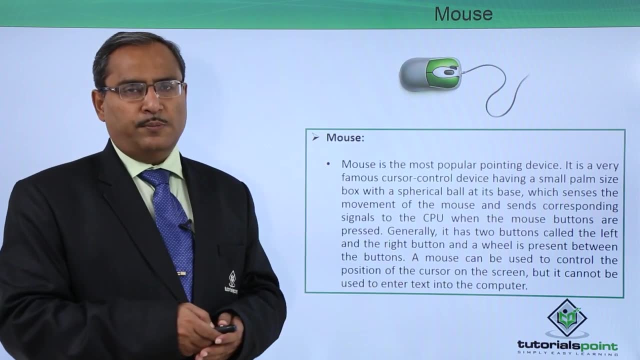 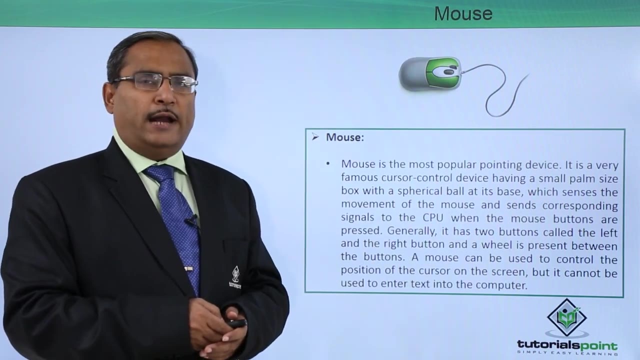 be used to enter the text into the computers. for that we usually use our keyboards. So this is the. this is the description. whatever we have given here is known as the ball mouse, but now it is. we do not use the ball mouse. The ball mouse usage is very rare. we use optical mouse and also we use wireless. 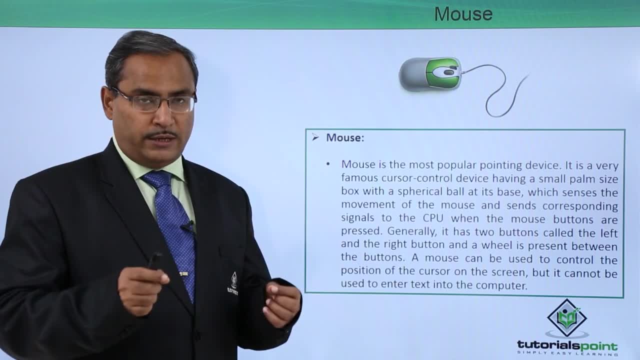 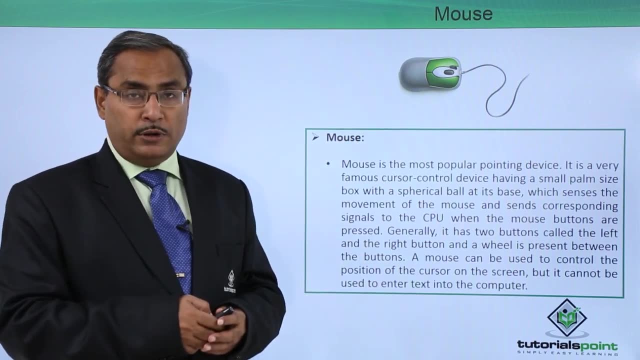 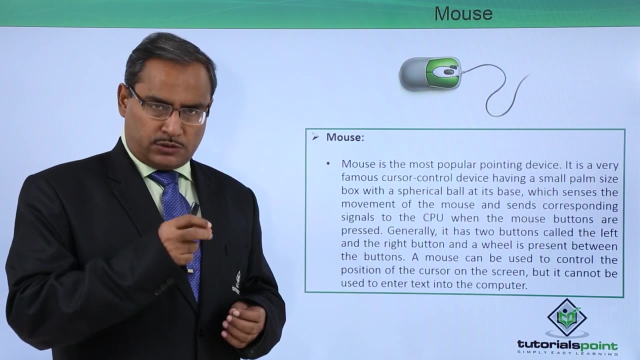 mouse, The. that is no connection, there is no where in between the respective laptop or the CPU and with the mouse. So that is the wireless mouse are very common nowadays in use and also the optical mouse, And here we are having two buttons. we can click on those buttons. there is one scroll. 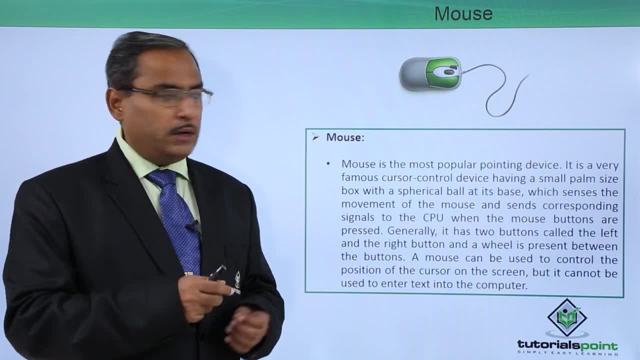 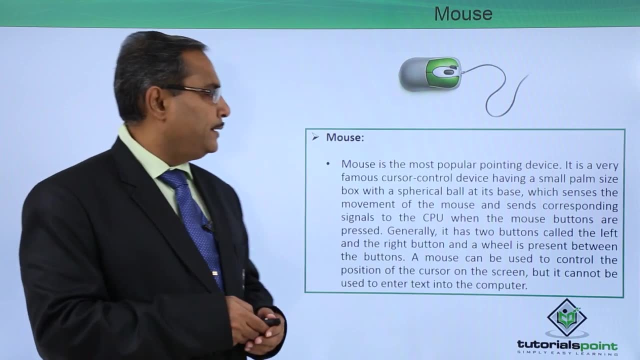 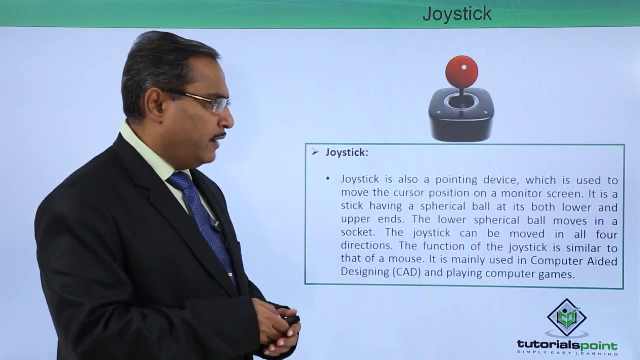 is there. in between those, one wheel is there, So we can roll that one and in this way we can control the resolution of the mouse respective cursor movement and pointer movement on the screen. Now let us next one is about joystick. So joystick is also a pointing device, which is 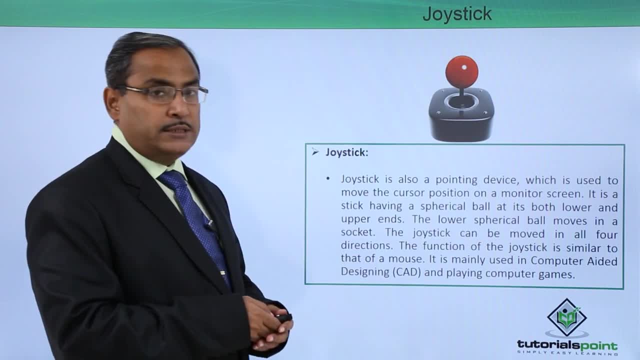 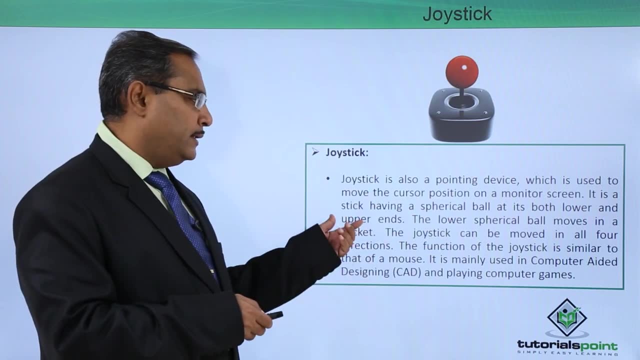 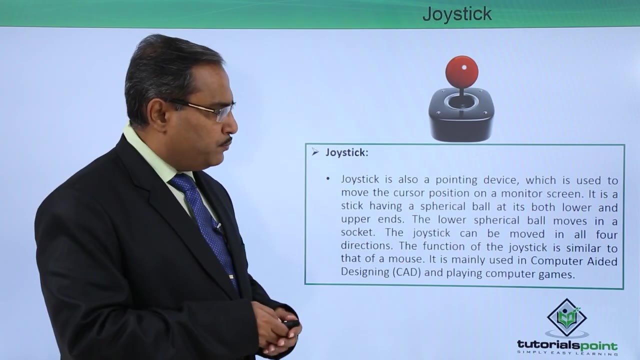 used to move the cursor position on a monitor screen And it is a stick having a spherical ball at its both lower and the upper ends And the lower spherical ball moves in a socket. The joystick can be moved in all four directions. The functions of the joystick is similar to 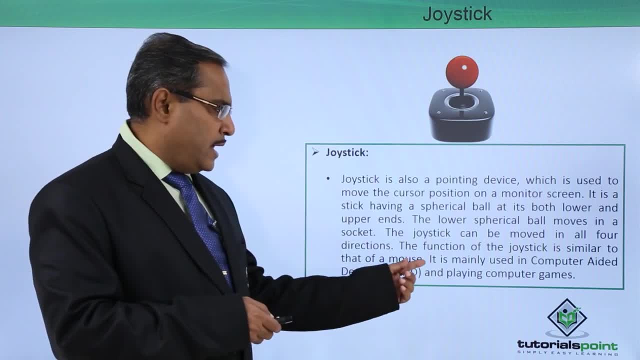 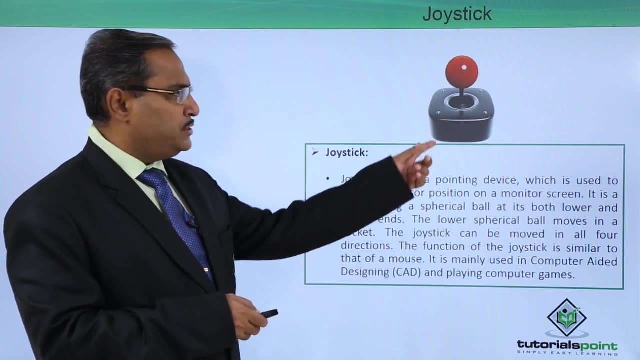 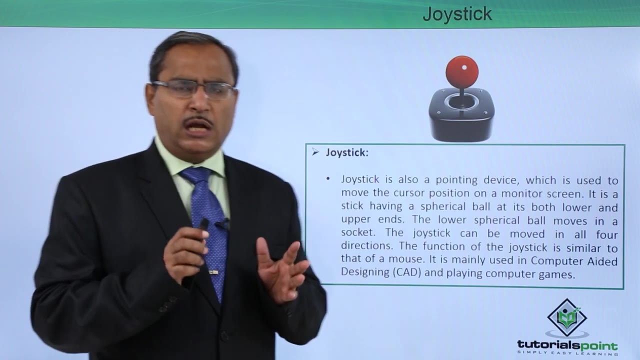 that of the mouse to change the position of the pointer, And it is mainly used in computer aided designing, CAD and playing computer games. So this is known as the joystick. Here we have given one diagram on picture of joystick, So that joystick is not very much commonly.